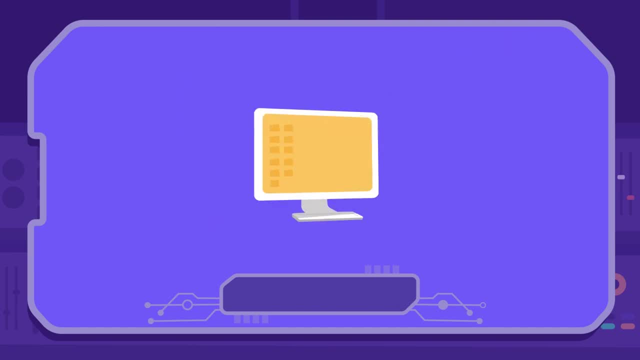 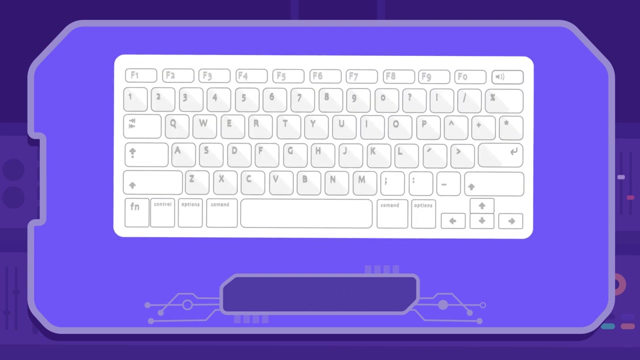 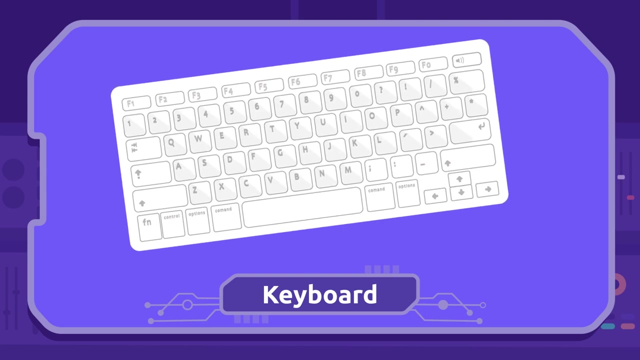 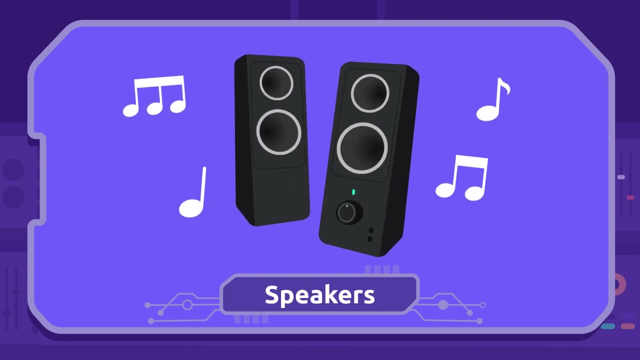 Computer Monitor: The monitor allows us to see images and computer data. Monitor Mouse: We use the mouse to select items and move the cursor on the screen. Mouse Keyboard: We use the keyboard to type. Keyboards have all the letter and number keys. Keyboard Speakers. 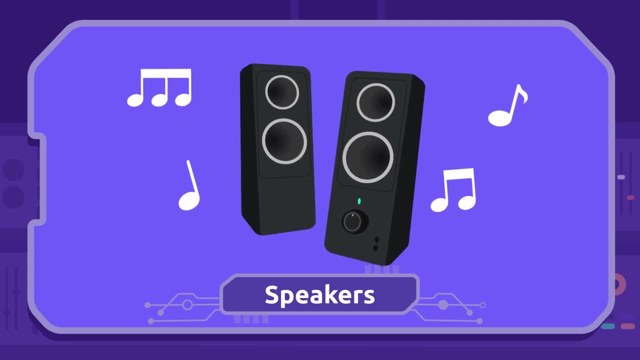 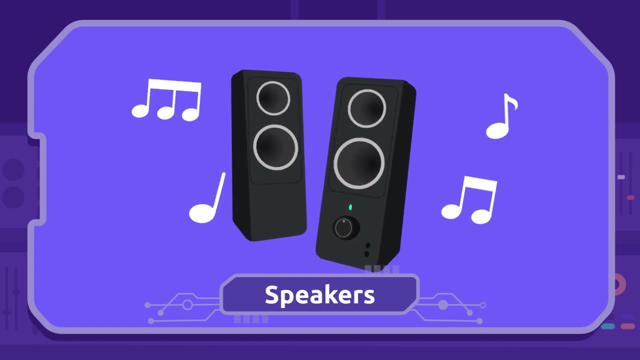 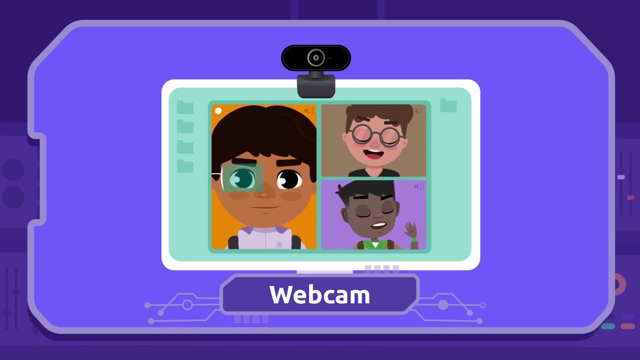 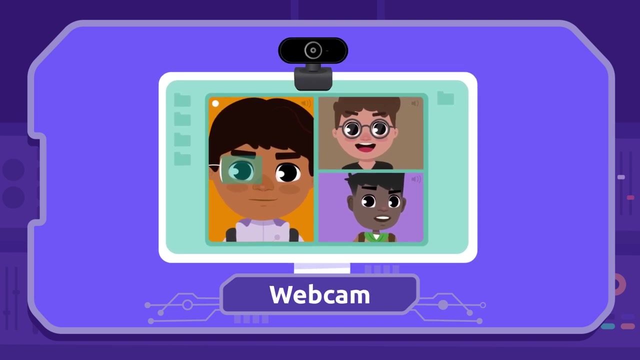 We play music and sounds through the speakers. I love this song. Speakers Webcam. We use the webcam to see each other on the screen. Thanks to the webcam, we can make video calls to see our friends and family. Webcam Webcam, Webcam- Webcam- Webcam Webcam. 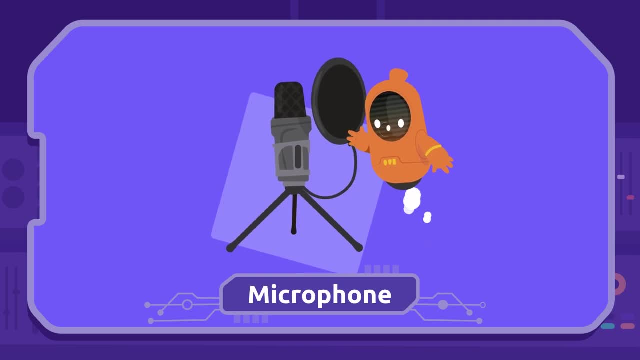 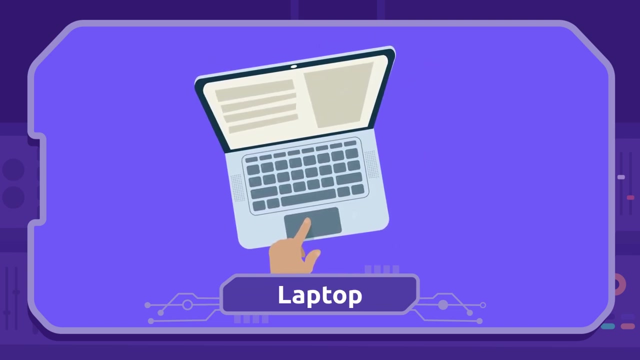 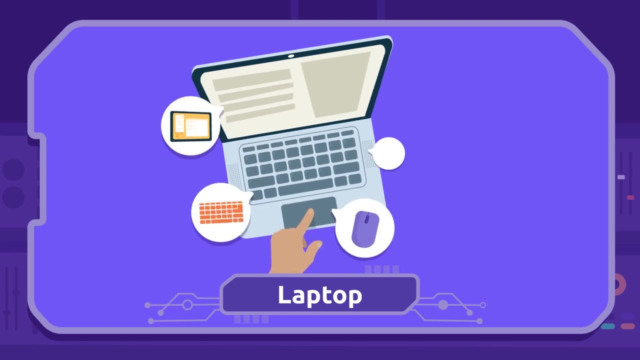 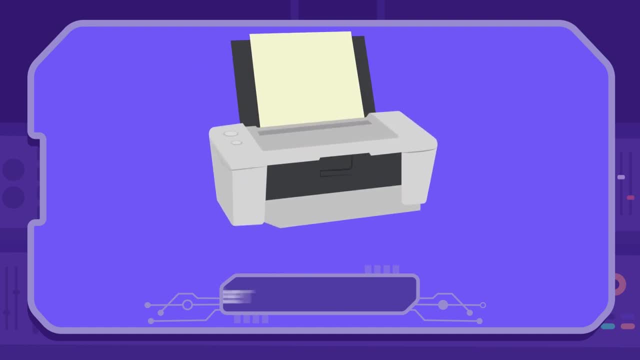 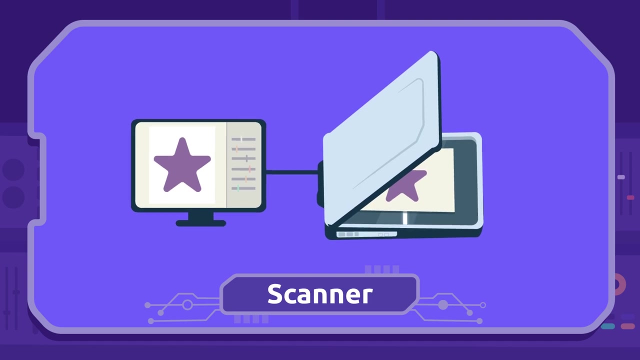 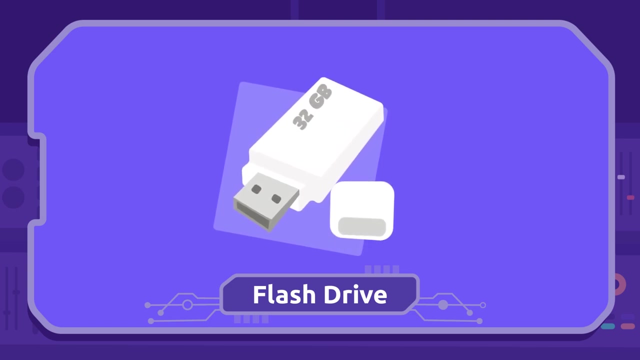 Laptop Printer: We use the printer to put on paper text and images from the computer. This is called printing Printer. Scanner: We use the scanner to pass documents and images from paper to the computer. Scanner Flash drive: We use the flash drive to save files and copy them from one computer to another.